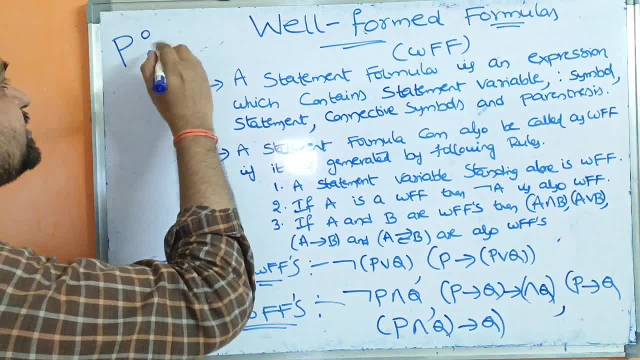 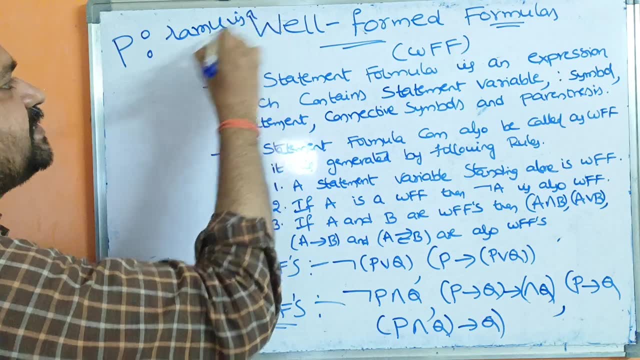 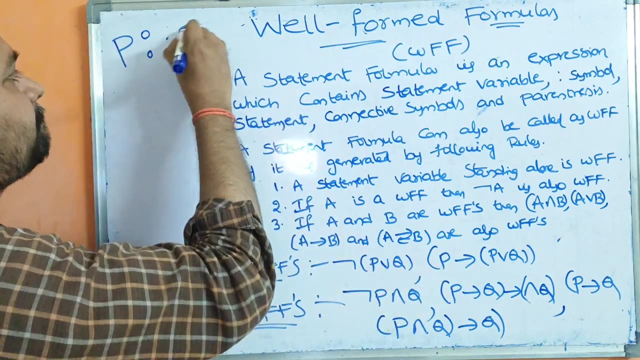 And a statement. Let us take a statement. Ramu is a good boy. Or we can consider any statement like PRQ also. There is no problem. So Ramu is a good boy. Likewise, we can take any statement. So let us take normal statements. PRQ. PRQ. Colon symbol, statement, connective 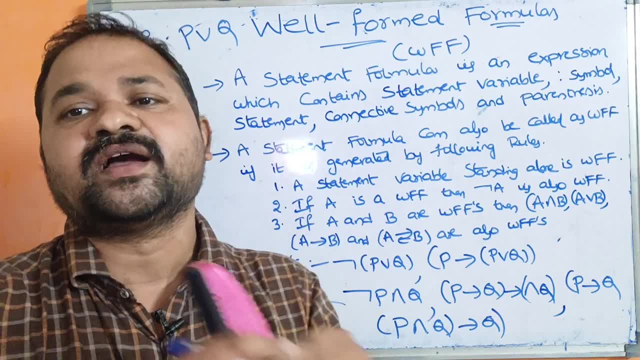 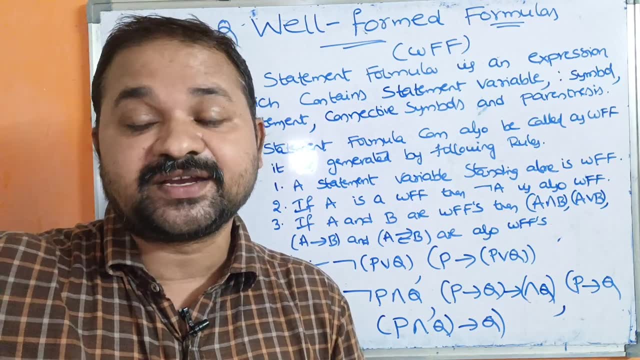 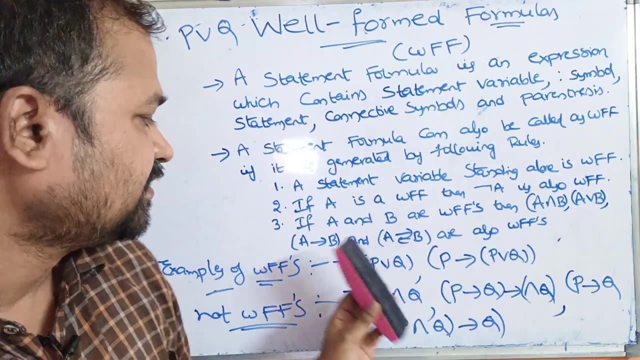 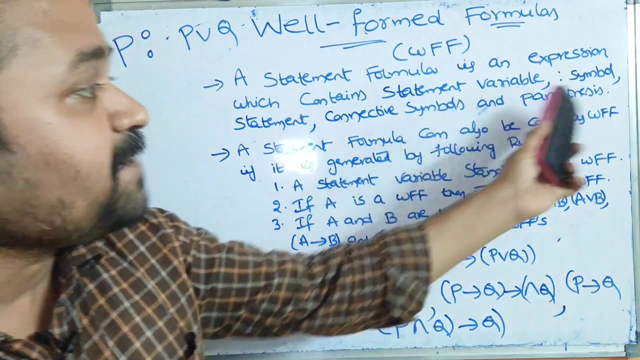 symbols. So statement formula means it should contain connective symbol. We have five connectives are there. Under connective, conjunction, or connective, disjunction, or negation, next implication, implication. This is implication. Next conditional. Next biconditional. So statement formula must contain a connective. And parenthesis symbol. So it should be placed in parenthesis symbol. 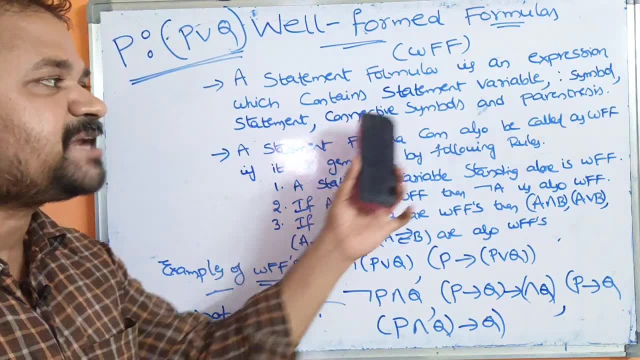 So this is called as statement formula. A statement formula is an expression which contains a statement variable. Here P is called a statement variable. 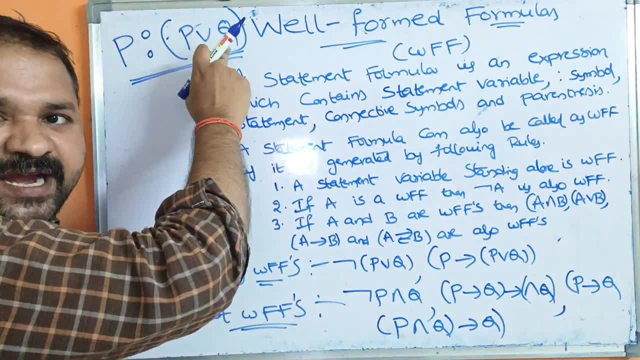 Colon symbol. And it contains some statements. Here P and Q are called as statements or propositions as well as connectives. As well as connectives. R is connective. 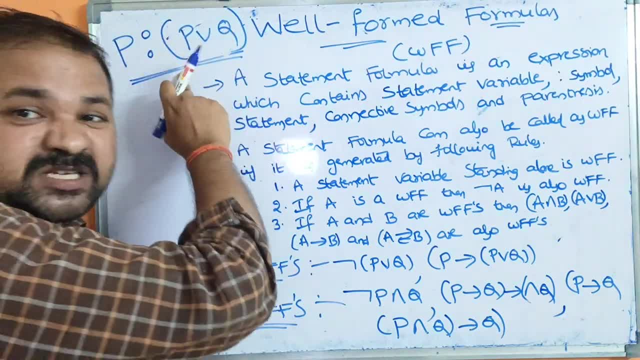 And parenthesis. This formula, statement formula, must be enclosed in the parenthesis symbol. Must be enclosed in the parenthesis symbol. 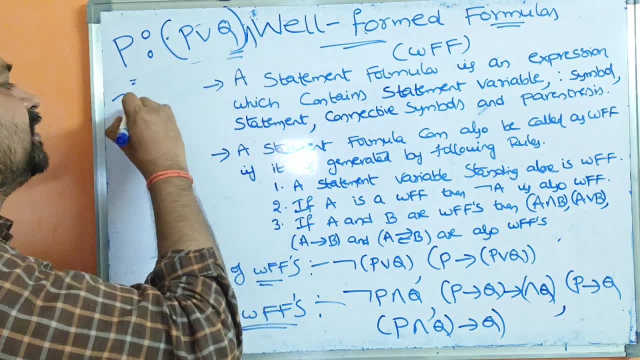 Likewise, we can take a number of statement formula and negation P or Q. So this is another 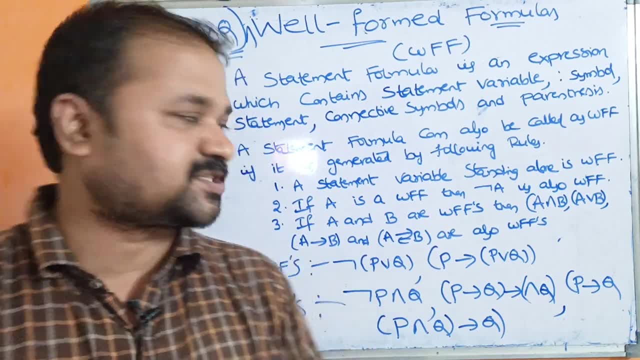 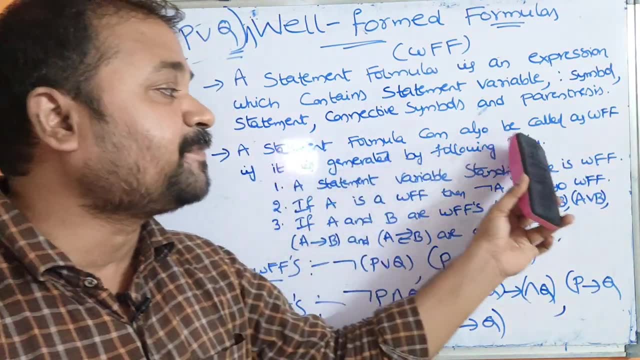 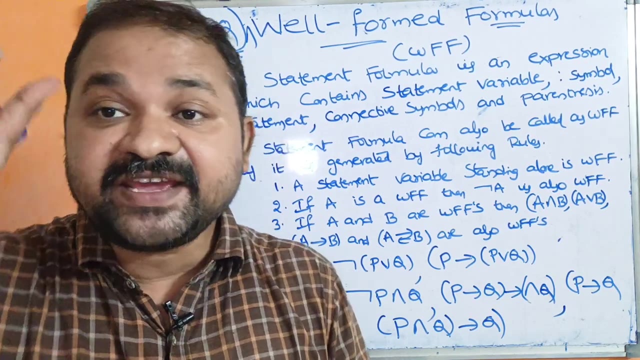 statement formula. So likewise, we can take n number of statement formulas. A statement formula can also be called as well-formed formula if it is generated by the following rules. So, we can call a statement formula as well-formed formula also. When we can call statement formula as well-formed formula? If well-formed formula 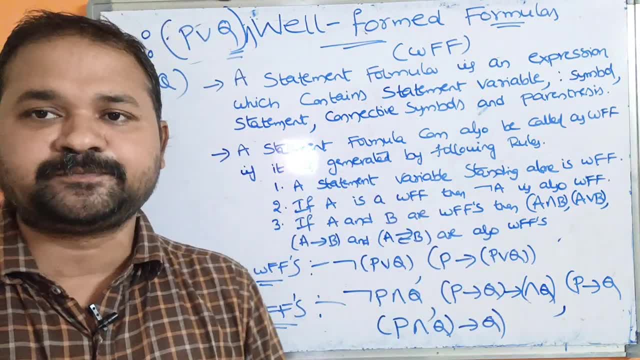 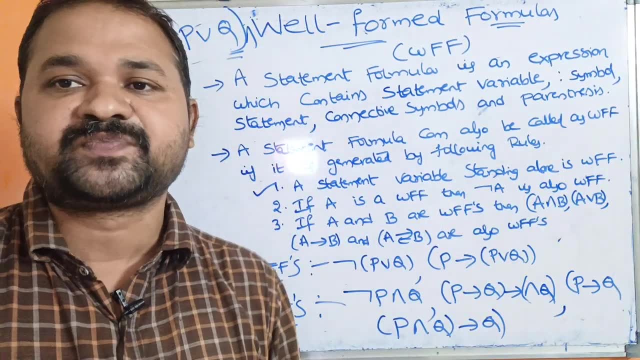 is generated by following these three rules. The first rule is a statement variable standing alone is a well-formed formula. A statement variable standing alone is a well-formed formula. 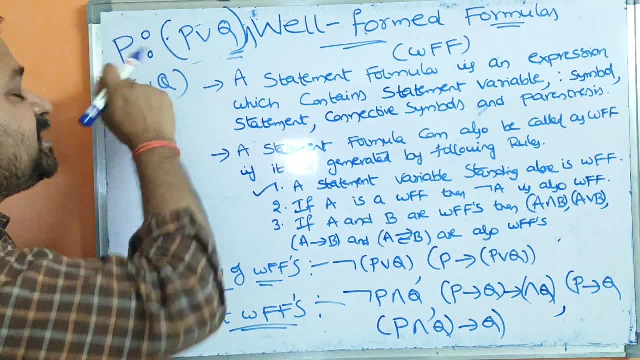 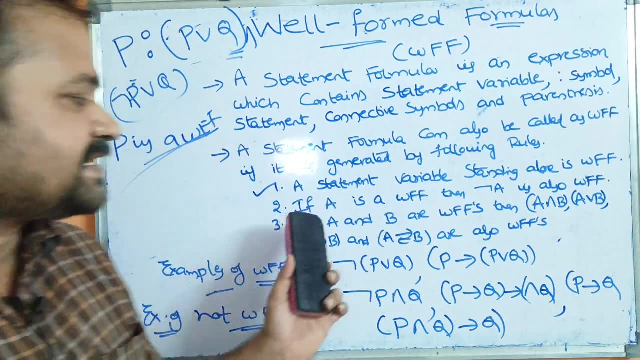 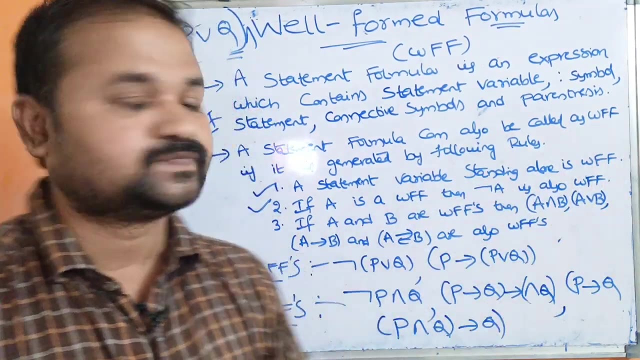 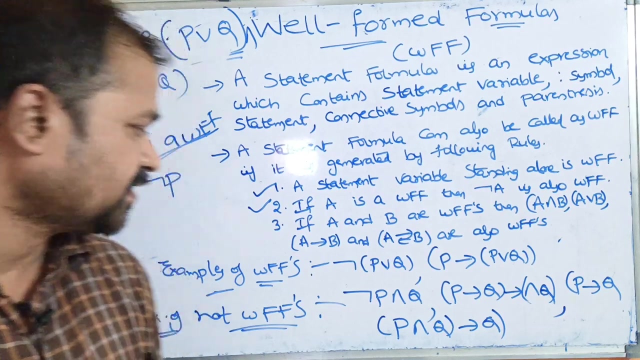 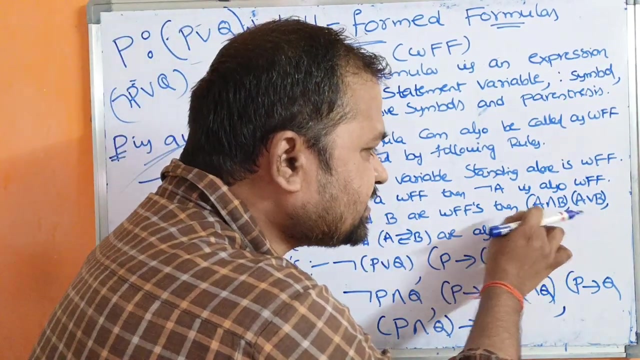 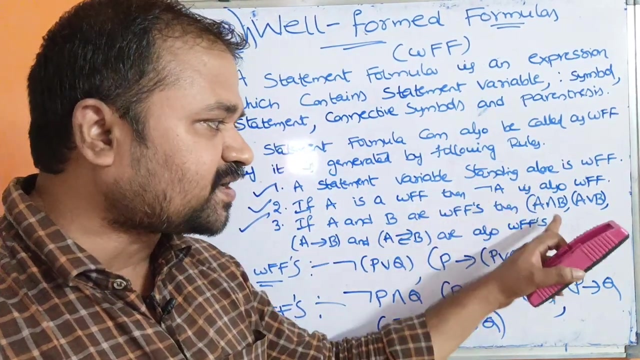 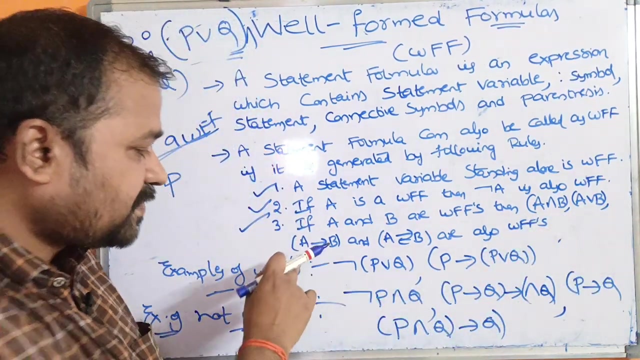 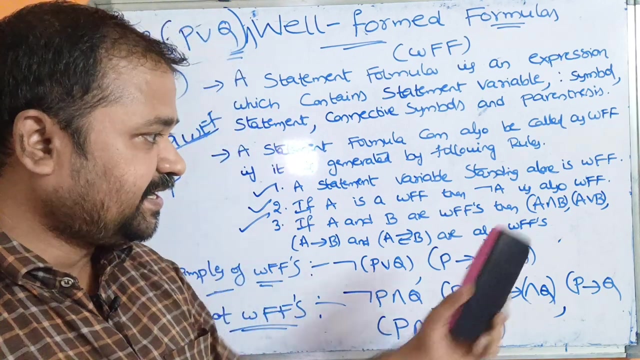 Here we have a statement formula like this. Here what is the statement variable p? So, p is a well-formed formula. p itself is called as a well-formed formula. Let us see the second rule. If a is a well-formed formula, then negation a is also well-formed formula. So, if p is a well-formed formula, then negation p is also called as well-formed formula. And the next rule is if a and b are well-formed formulas, then this is a statement formula. So, we have to enclose this in the parenthesis. We have five connectives are there. All the negation is over. The remaining four are a and b. We have to enclose in parenthesis a or b. Next, a implies b, a conditional b and a biconditional b are also called as well-formed formulas. Here we have to enclose them. 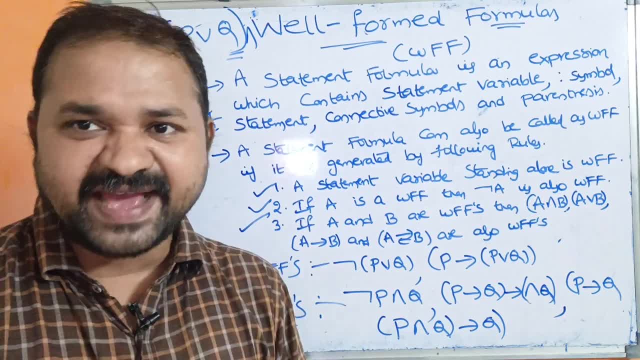 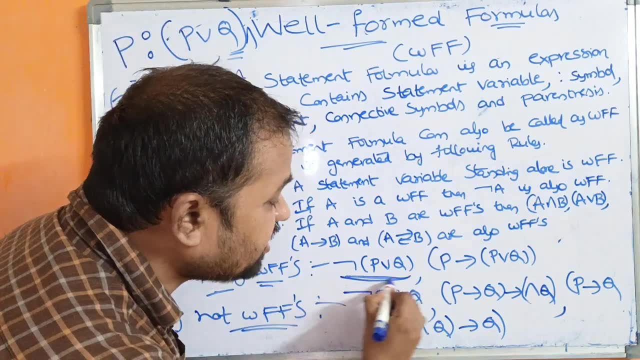 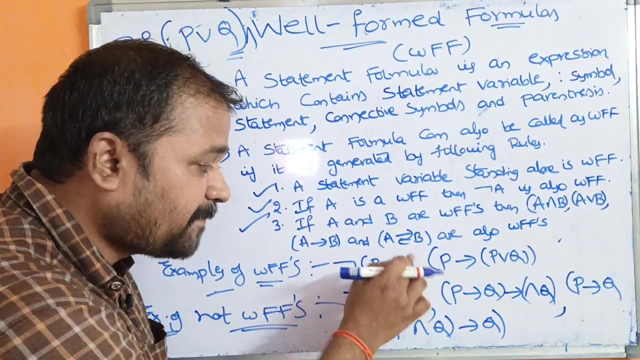 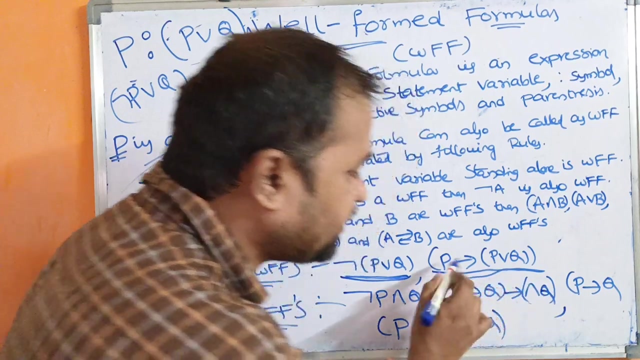 In parenthesis. Now, let us take the examples of well-formed formula and not well-formed formulas. Negation of p and q. Negation of prq. So, this is a well-formed formula. This is a well-formed formula. Why? Because here we have parenthesis symbol as well as we have connectives also there. Next, if you consider this one, p implies prq. Here prq is enclosed in the parenthesis next to p implies prq. 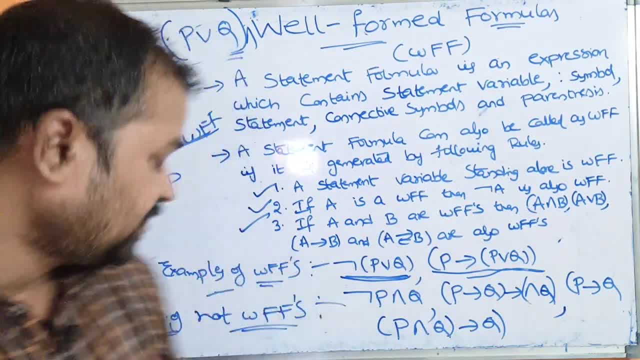 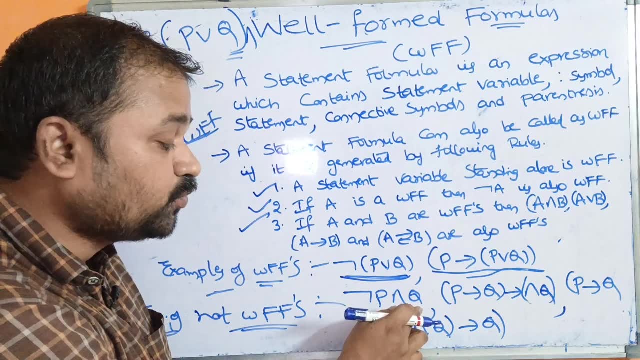 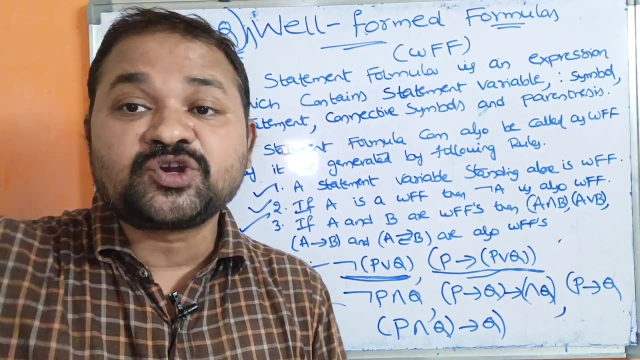 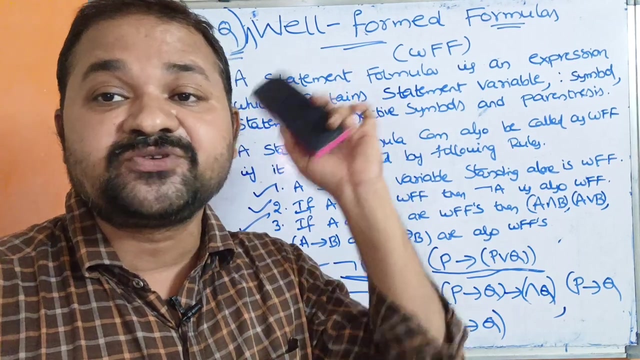 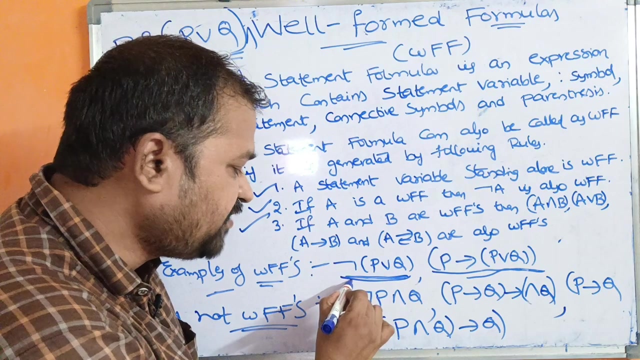 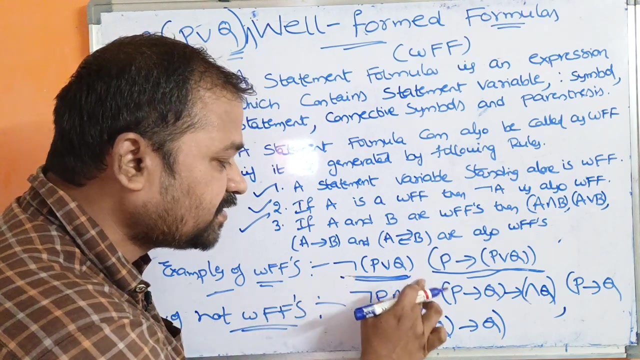 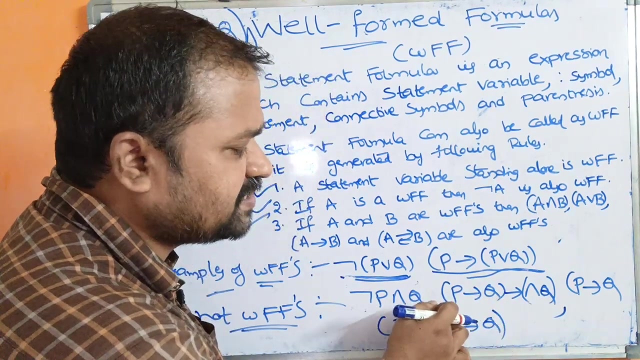 So, this is also a well-formed formula. Now, let us see the examples of not well-formed formula. Negation p and q. Negation p and q. This is not a well-formed formula. This is not a well-formed formula. Why? Because well-formed formula means it should be enclosed within the parenthesis. A statement formula is called as well-formed formula. What is a statement formula? We must use the parenthesis symbol. Here we did not use any parenthesis symbol. So, that is why this is called as not well-formed formula. So, this is not a statement formula. If we enclose within the parenthesis, then it can be called as well-formed formula. But in this example, we do not have parenthesis symbol. So, that is why this is not well-formed formula. Let us see this example. p implies q. Very good. This is enclosed in the parenthesis. Implies. But here we have undies there. Undies performed on two statements. 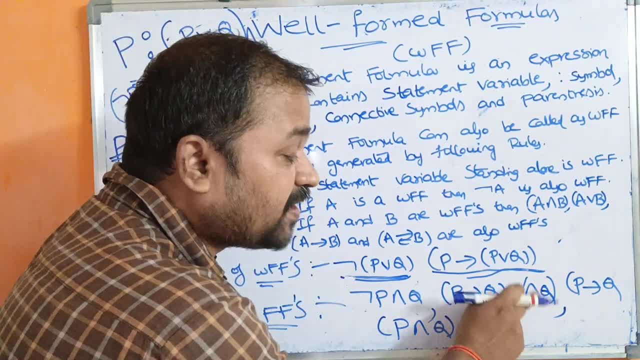 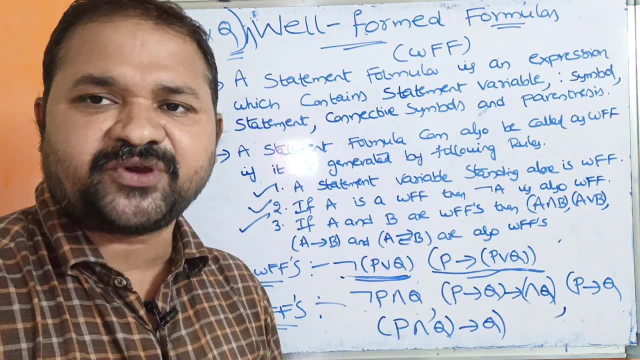 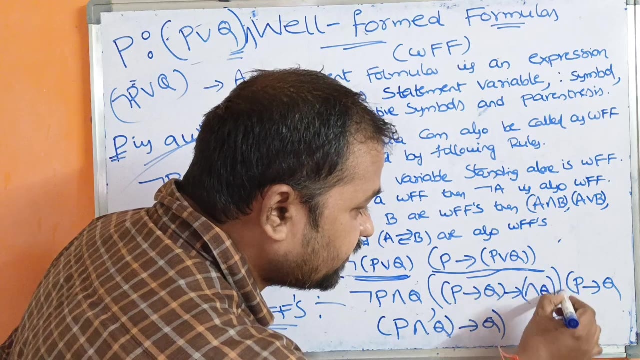 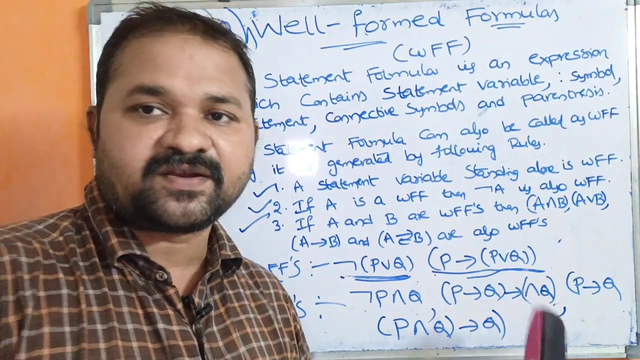 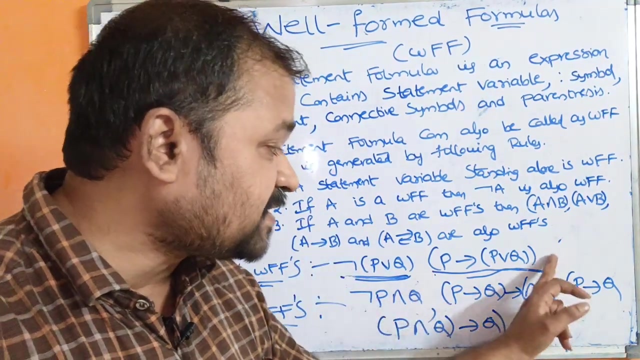 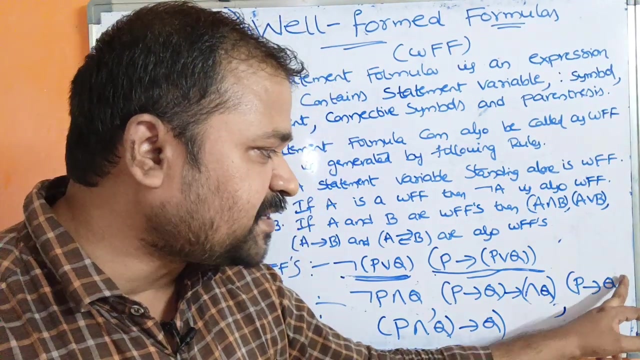 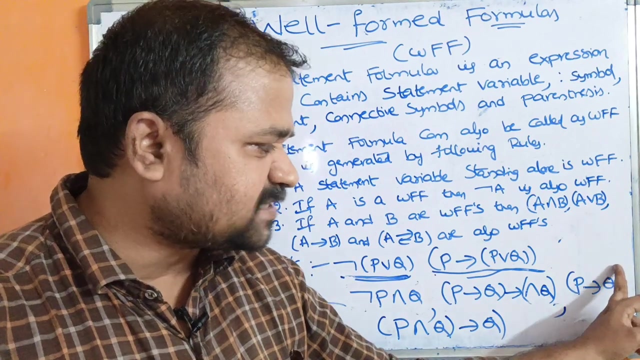 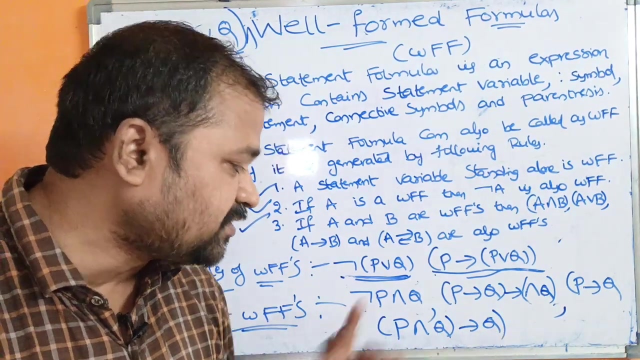 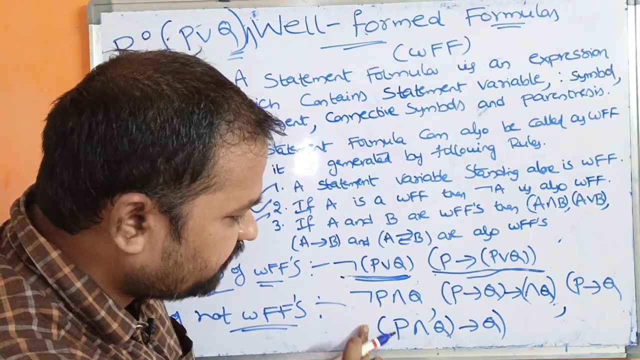 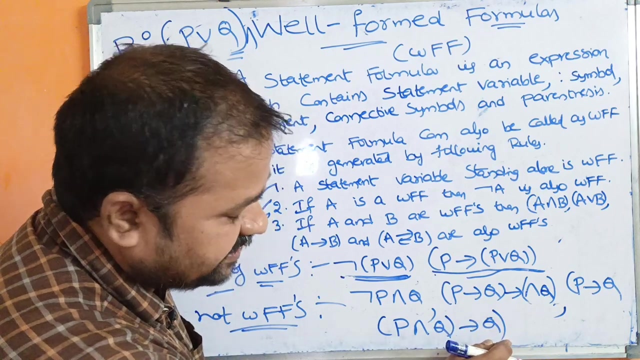 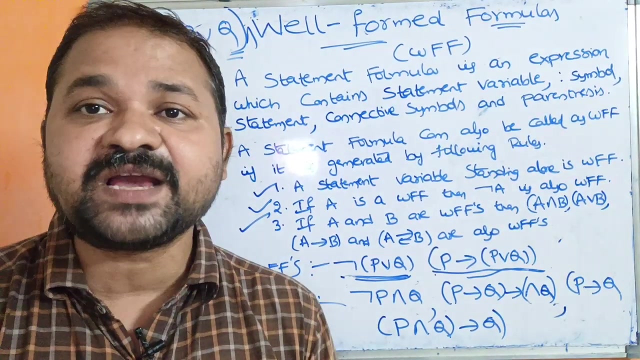 Undies performed on two propositions. But here we have only one proposition is there. We do not have another proposition. Here we may have either. p or any other proposition. So, that is why this is not a well-formed formula. As well as here, we do not have parenthesis symbol here. We do not have parenthesis symbol. So, that is another reason why we are not calling this as statement formula. Here we have two mistakes are there. Beforehand, we must require one more statement or one more proposition and this entire expression should be enclosed in the parenthesis. Let us take this example. This is also not a statement formula. Why? Because in this expression, right parenthesis is missing. If we have right parenthesis, then it will become a statement formula. But this expression does not contain any right parenthesis. So, this is not a well-formed formula. If we consider this one, p and q implies q. This is also not a well-formed formula. Why? Because here, the left parenthesis is missing. We do not have the left parenthesis. p and q, very good. It is enclosed in the parenthesis. Implication q. Here, right parenthesis is there. But left parenthesis is not there. So, this is not a well-formed formula. So, this is about well-formed formulas. 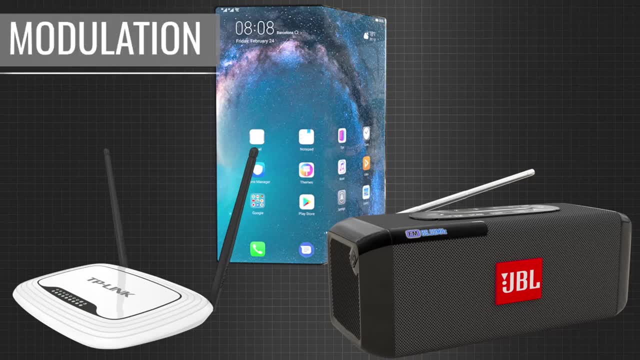 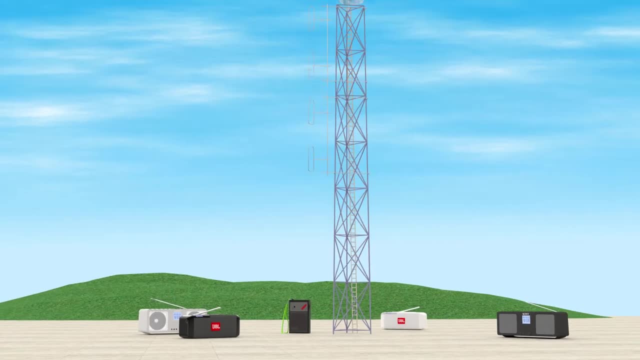 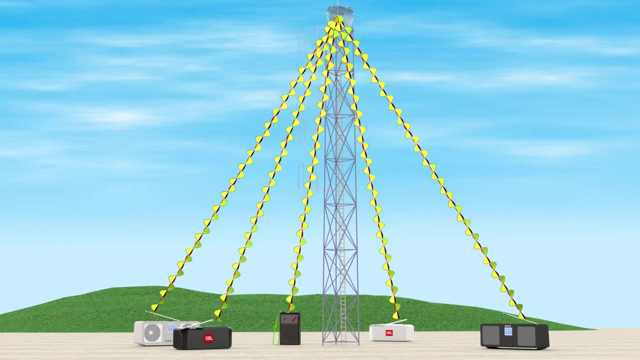 Modulation is one of the most frequently used technical words in communications technology. One good example is that of your FM radio, where FM stands for frequency modulation. In this video, we are going to learn the basics of modulation techniques and see how they are applied in modern cellular and communications technology. 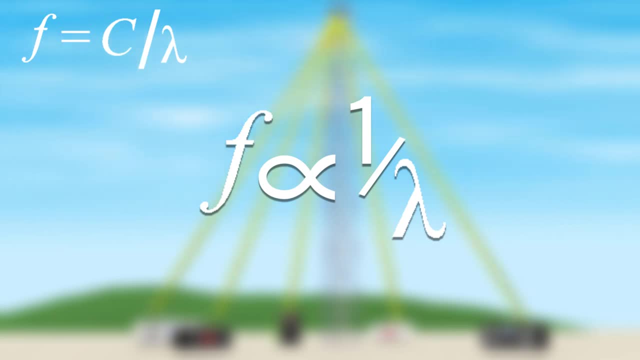 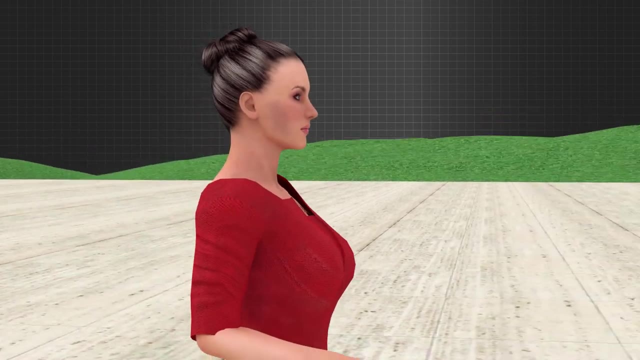 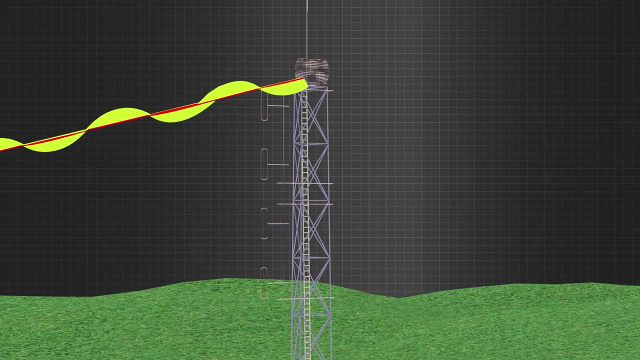 Frequency and wavelength of a wave are inversely connected. Humans have the capability to hear sound frequency from 20 Hz to 20 kHz, but if a radio tower transmits electromagnetic waves of the same frequency, the size of the antennas required will be really high. In the antenna video we have already seen that the size of the antenna is. 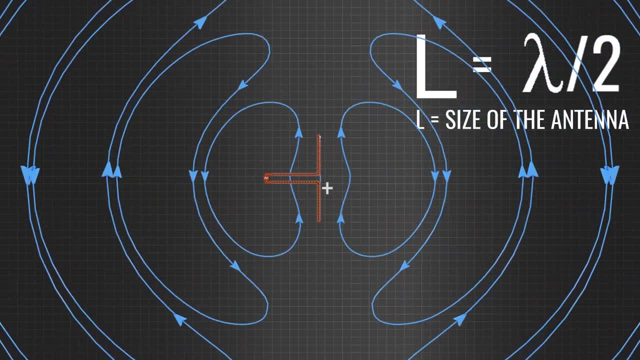 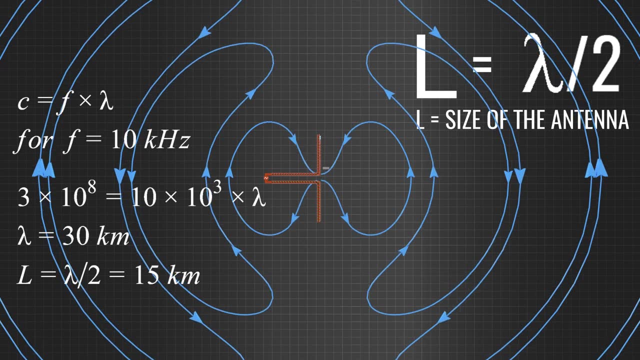 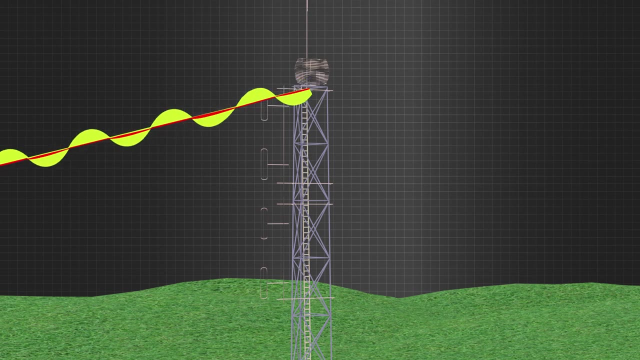 proportional to the wavelength. If we had transmitted the electromagnetic wave in the same frequency of sound, the antenna size required would have been in the range of kilometers. This is why we need modulation. Before the electromagnetic waves are transmitted, they should be modulated to a high-frequency signal.